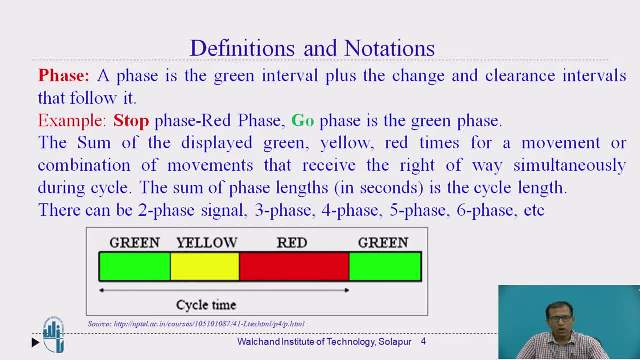 So after the cycle we must know what is a phase. So phase is the green interval plus the change and clearance intervals and that follows it. So here we are going to use the stop phase, that is, red phase is called as a stop phase and go phase is called as a green phase and clearance is indicated by yellow indications. 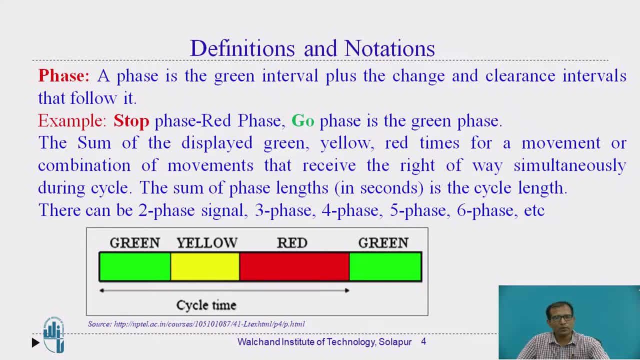 So the sum of the displayed green, yellow and red- And that decides whether it is the one con goodness or the other one- is of no İsacă benefit. So the initial state is in the second stage of the cycle course types, which are that one. 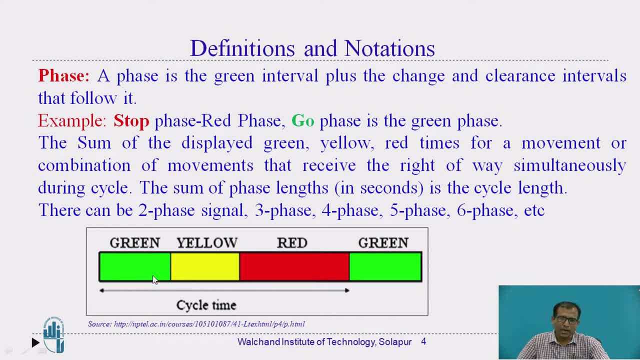 Ah, but you can come up with another. Er. there is also another way that I have notice. It is to know that is a variable atta or less number of the phases are feasible, So the one phase indicates the all green. 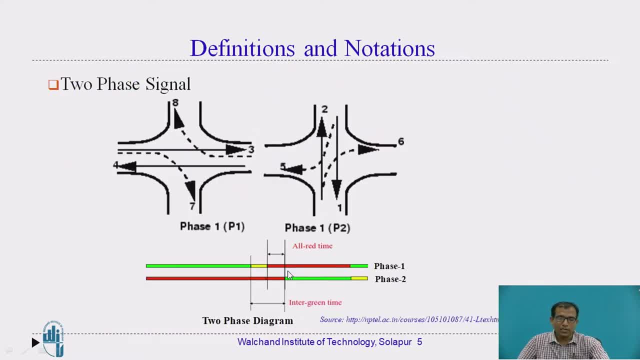 yellow and red phases. So let us understand this phases in detail. So this is the two phase signal. What is two phase? In the first phase, you see that the four moments are allowed. It means, while giving the green to this moments in first phase, the green is given to this. 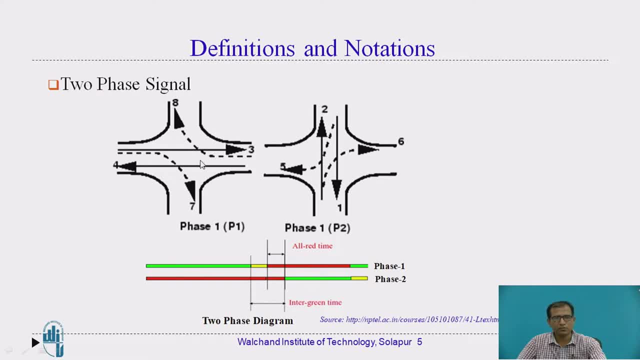 the first, the location- This is for the moment of the straight moment, and this moment- and also there is a turning moment- is also there. There is a right turning and left turning moment. So in one phase, all this four directions are cleared and after this, once this phase, 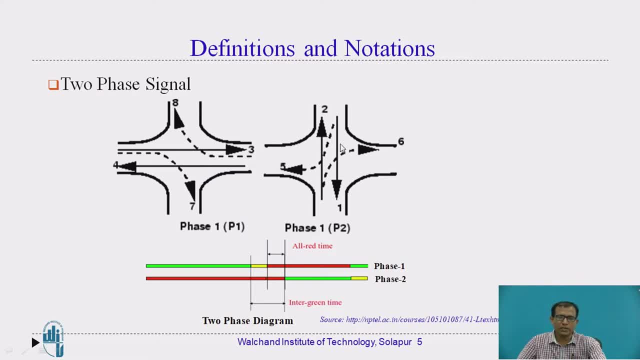 is over. the green is over. If you are going to get the second phase, this is for the another side. you are going to get the another phase. So for this we are going to put the red and we will operate this green for the second phase. So again, the another four directions are cleared in. 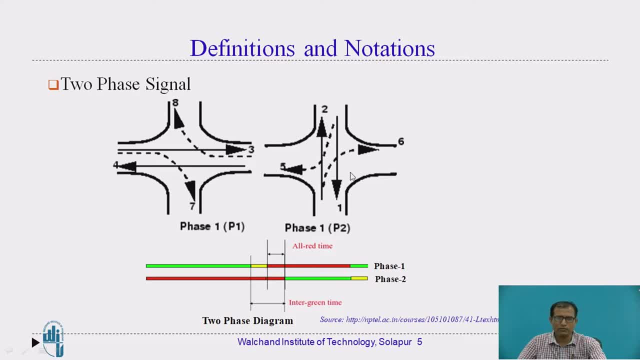 the second phase. So straight moment and also left turn and right turn moment. So it is very difficult if the right turning moment, left turning moment is there in one phase. So it is very difficult to clear this moment because while taking the turn 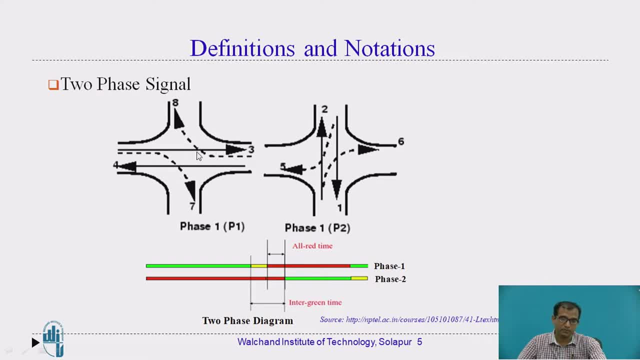 you can see here there is a congestion point or conflict point over here. So here is one conflict point, another is a conflict point. So this has to be decided. basis on the geometry of the intersection: how much area is available, what is the traffic intensity? On basis of: 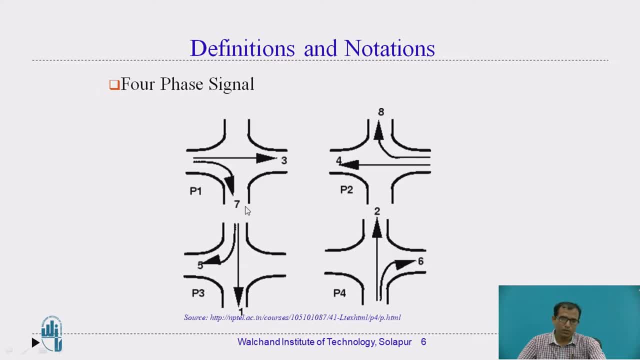 this number of the phases are decided. So this is the four phase signal. So in this one you can see that same four leg intersection. We are operating two, two directions. one, So means one, phase means one. green. So by giving 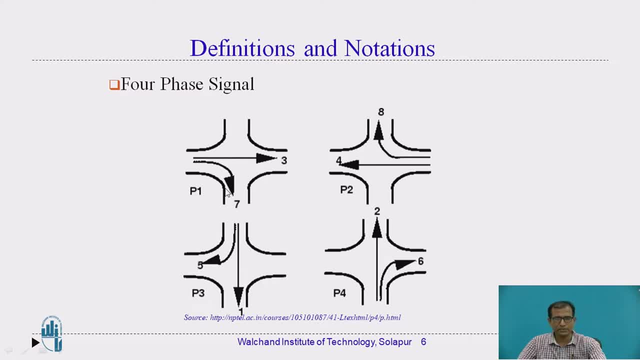 the one green. they are trying to clear seven and three directions and in second point eight and four directions are cleared. So it means this four leg is operated, four greens or the four complete rotation of green, amber and red signal. So this is the four leg intersection. 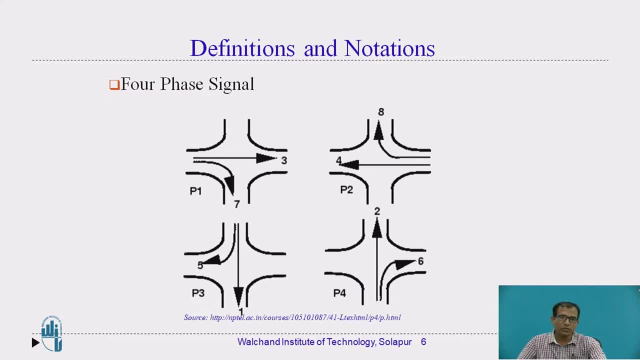 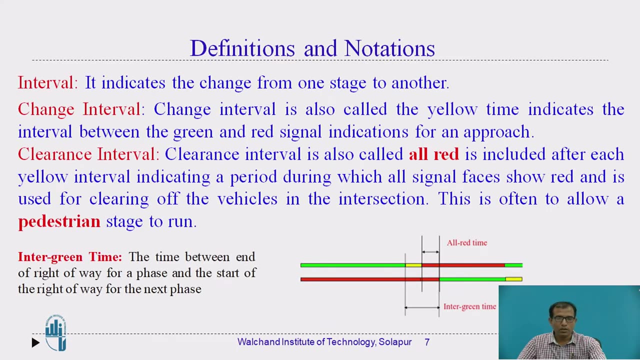 and four phases. More the number of the phases is increases means you have to the waiting period of the particular location will get increases. So we should note down that more the number, more the waiting period or the more the delay on other leg. So interval is the we have. 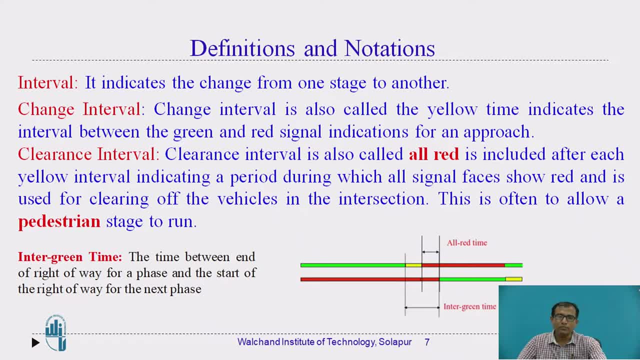 a two intervals, that is, a change interval and clearance interval. So change interval, it is the interval between the red and green signal. So that is, you can see that this part of the yellow is indicates the change interval. Clearance interval is given by all red time, So in this one all red time. 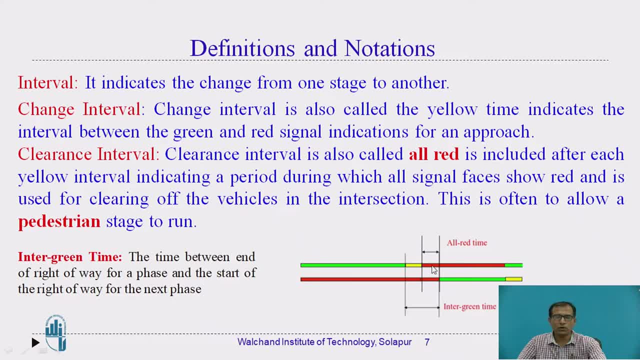 we can see that the all red is used for clearing pedestrians, clearing emergency vehicles, and if there is vehicle still, he is continued in the yellow phase and still there in the. he is at the mid of the junction, or at the dilemma location or at the mid of the junction. 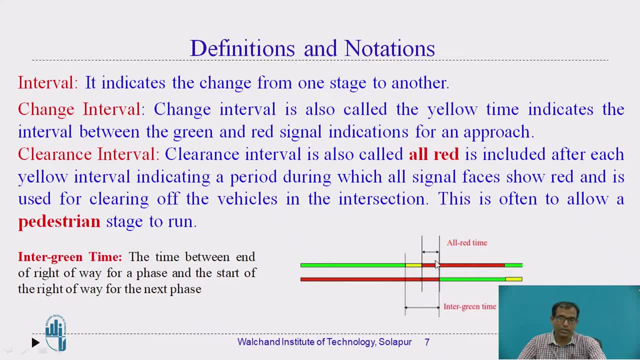 still that particular vehicle is not cleared, We can use that clear this all red time, clear that vehicle in all red time, and once that the all the clearance is done, then we can give the green for the next leg. So otherwise you may end up with the accident also. 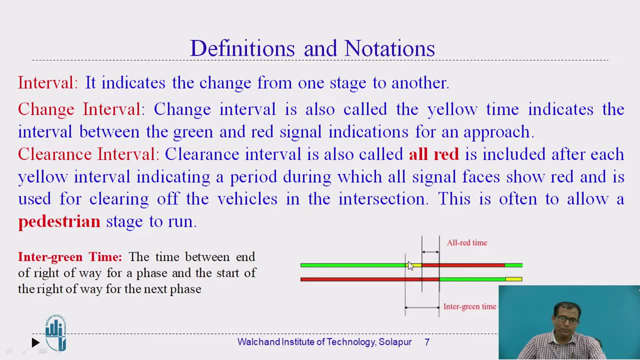 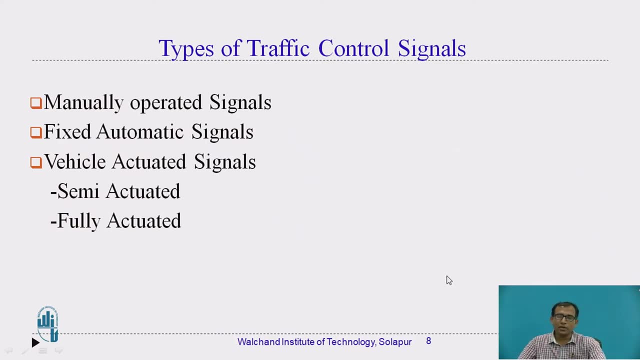 So another term: inter green period. End of the green period. The green to the start of the another green is called as a inter green period. So this includes the change interval plus all red time also. So this is the inter green period. Now we have different types of the signals: Manually operated signals, fixed and vehicle. 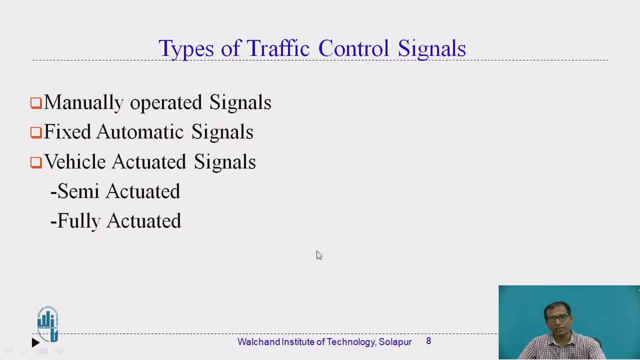 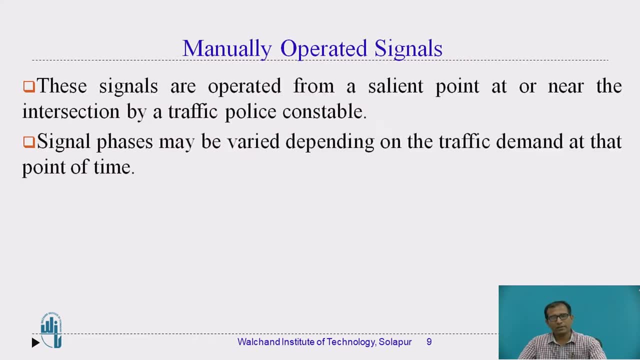 actuated signals. So again, in that semi actuated and fully actuated signals, The first, we will see the manually operated signals. So this is. everybody know that this is the particular signal operated by a traffic police and depending upon the availability of the traffic police he is going to and demand, depending upon the demand of the particular, 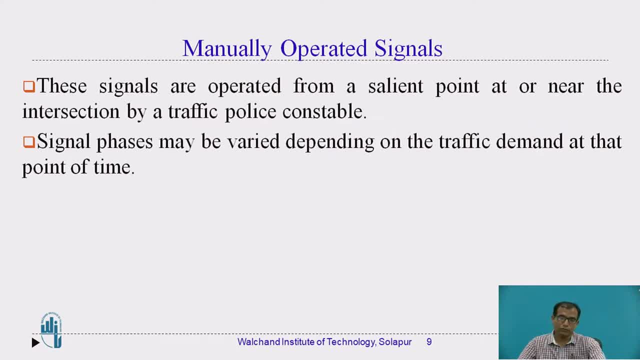 traffic intensity, he will change the timings. also, If there is no vehicle are there in the particular leg, he may put the that particular leg as a red, So like this. but the drawback of the system is what happens if the traffic police is not there, If the vehicle is not. 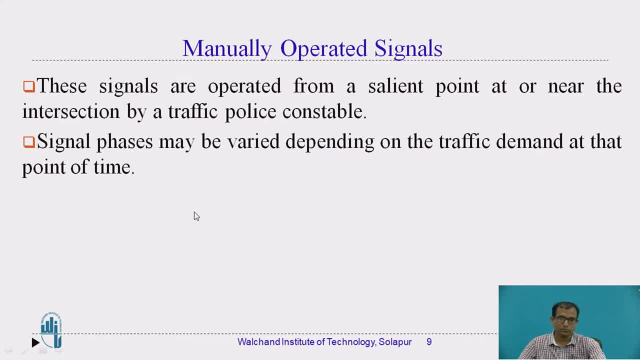 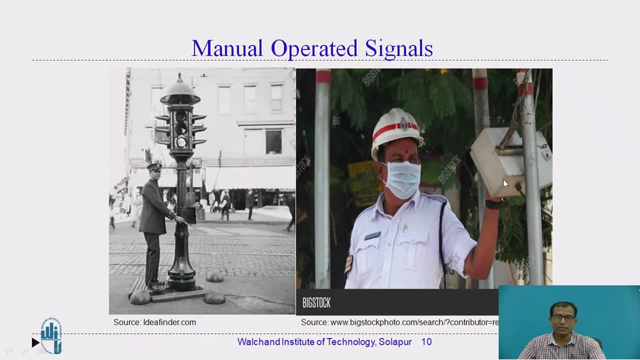 there cannot move toward the��. that is the drawback of the manually operated signals. So this is the picture. We try to operate the signal boxes there, So traffic police will come and operate at the corner of the junction. So operating the, changing the different. 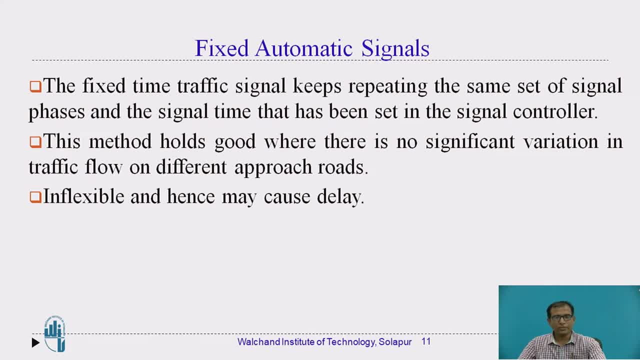 signal timings. Now, next one is a fixed automatic signal. In this one we going to fix the cycle length. The red, green and amber- all the timings vary. Sorry, this happens as they change the signal also, For example, again the red to green and amber, all the timings. we change the signal time since. 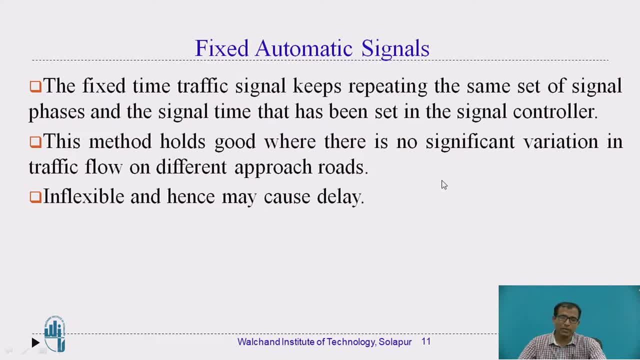 they fall out of the straight line on this track. So even in this thing we have to reduce the Midwayiked. So that means if you want to update the vehicle itself, or at least the maintenance, are fixed and this will change, the rotation will change and same timing will be continued. 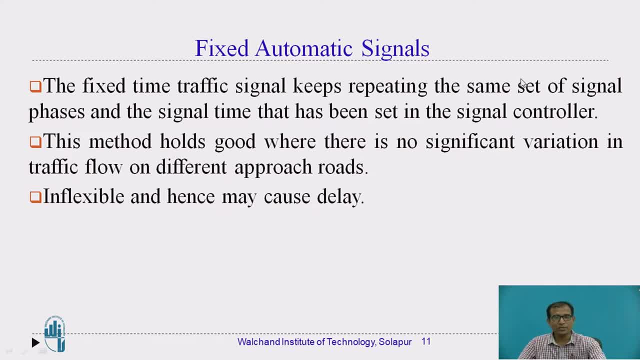 for all the legs repeating the same set of signal phases and signal time that has been set in the signal controller. So only problem is the inflexible and hence may cause delay Sometimes if there is no traffic is there at the particular leg. still we are going. 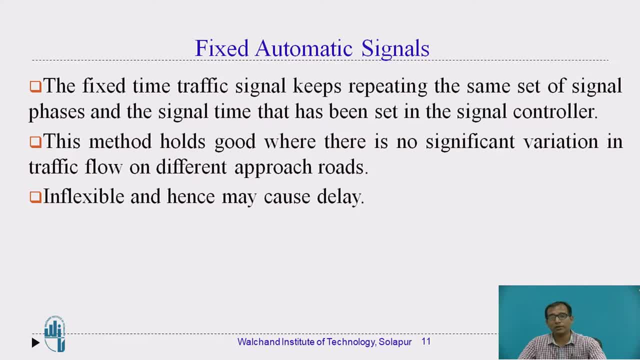 to operate red, green and amber The other, which are really required the green time. so that will cause a delay for the fixed automatic signal. So suppose the all the four leg has got a equal intensity of the traffic. in that case this fixed automatic signal will going to be very useful. 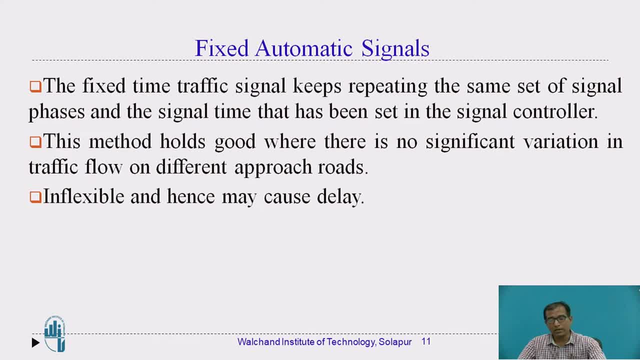 But if there is only some legs are having higher intensity and some legs are having no very less intensity Of the traffic and the signal timing which is going to operate on the those less intensity traffic may cause a delay to the other side which are really required: the green time. 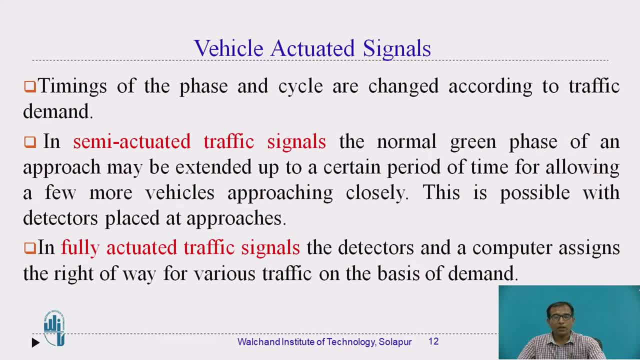 Hence it is inflexible and hence may cause the delay. Another one is the vehicle actuated signals. So we are going to use some detectors or sensors placed on the below the roads. So these we are going to, depending upon the type of the signal we are going to use, semi-actuated. 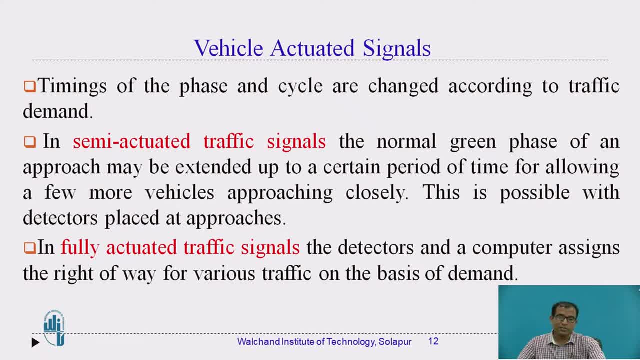 and fully actuated traffic signals. So here in the semi-actuated we are going to use this- detectors or sensors. The normal green phase of an approach may be extended up to a certain period of time for allowing a few more vehicles approaching closely. 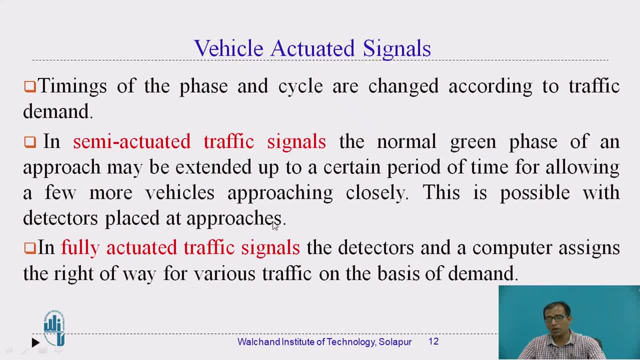 This is possible with detectors placed at the approaches. So one or two leg. we are going to use this semi-actuated traffic signals. Suppose the intensity of the traffic in all four legs are equal, So we are going to use this semi-actuated traffic signals. 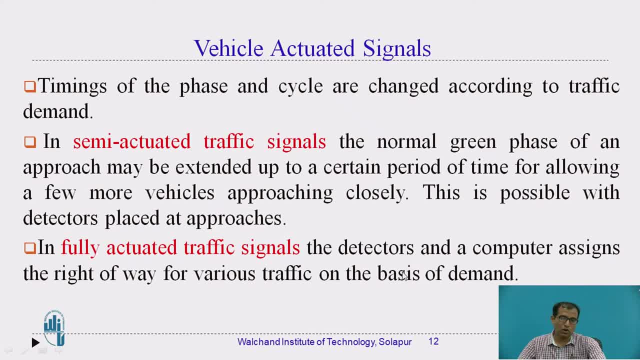 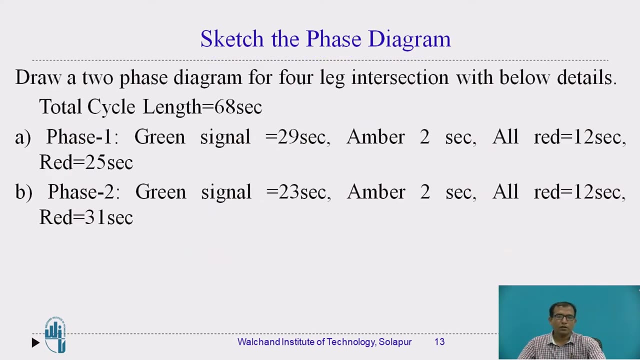 So all four leg has got the sensors and detectors and computer assigns the right of way for various traffic on the basis of the demand. So it is very useful but it is going to be costliest and depending upon the intensity of the traffic, these detectors will change the signal timings. 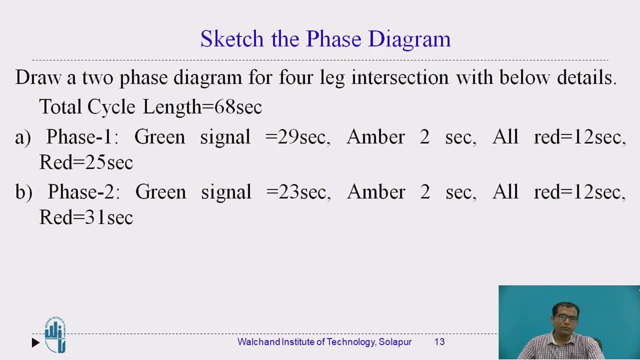 Now you can pass over here with understanding of the phase and the cycle. Here the total cycle length is given as 68 seconds to you. Here the total cycle length is given as 68 seconds to you and the green phase is given as 29 second. amber is 2 second and all red is given as 12 second and red.